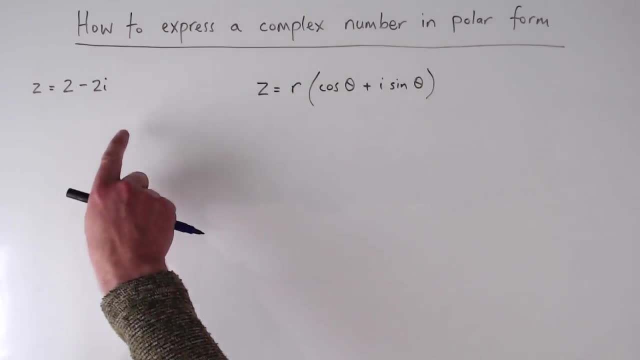 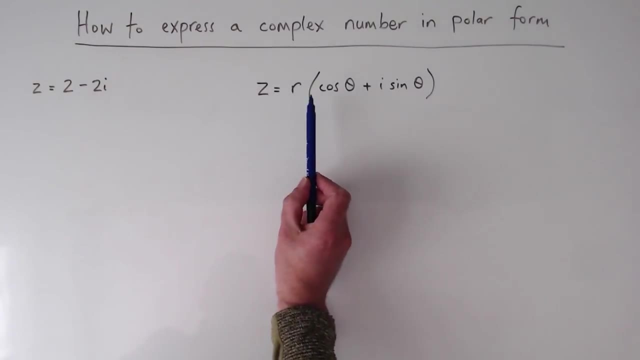 So at the end we can convert this back to Cartesian form and look at how they're interchangeable. So to do this, we need to take this number and we need to identify what the r component is, which is called the modulus, and we need to identify what the angle theta is called, its argument or its principal argument. 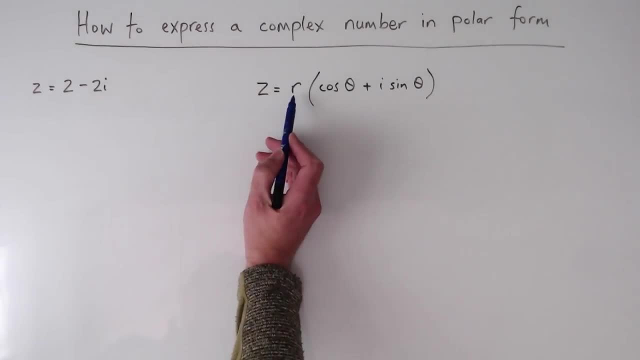 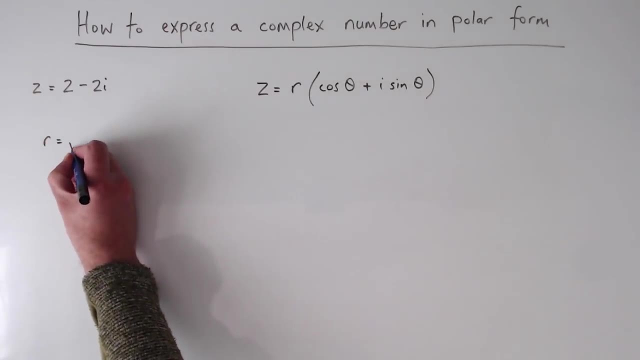 We're going to go through that process. Let's firstly calculate what the modulus is for this number, which is r. So r actually equals to the square root of this real component squared, so it is 2 squared, plus the imaginary part. squared, so it's plus minus 2 squared, okay. 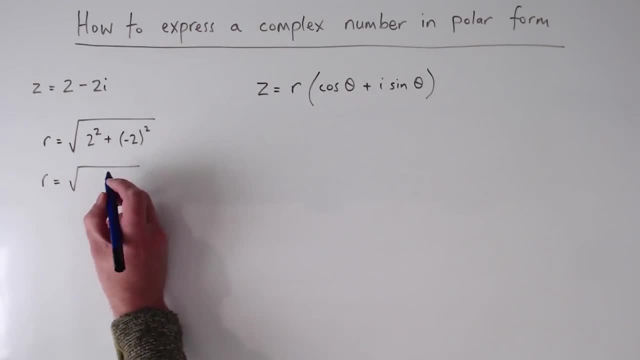 So if we work this through, that means that r would equal the square root of 4, 2 squared plus minus 2 squared plus 4.. So that equals the square root of 8.. Now to simplify this further, the square 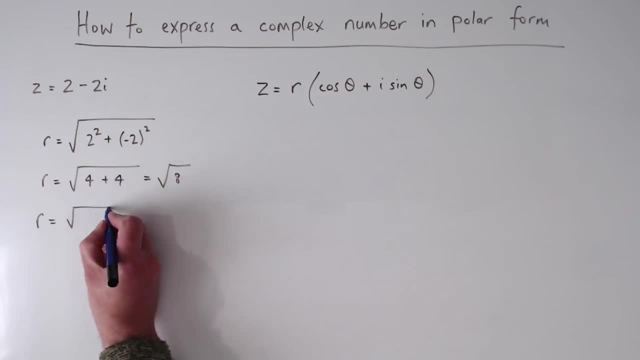 root of 8 can be written as 4 times 2.. I've done that because when I change the square root of 8 to 4 times 2, I have a square number here, so I can rewrite that as being r equals. 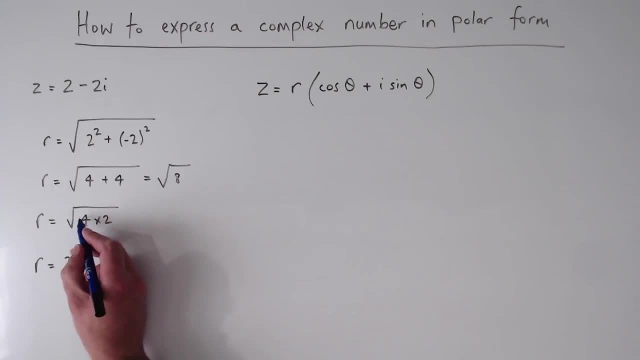 2.. We can take this square out: If here the square root of 4 is 2, 2 square root of 2.. Okay, So what we've done? by working out the modulus, we've got our first r component here. 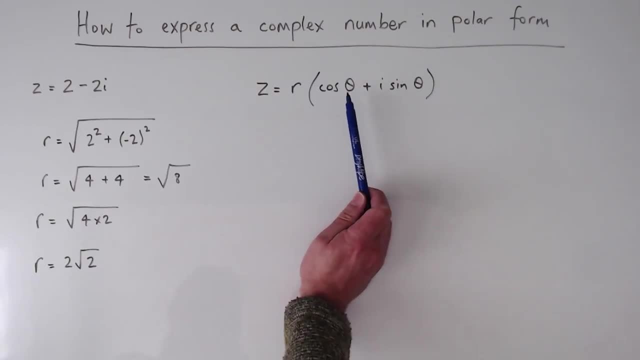 So we've done this part. We need to work out this angle, theta here, which they call the argument, And the way that we do. that is basically, if I have, if I, if I drew some axes, where this is the imaginary i-axis, this is my real component here. If 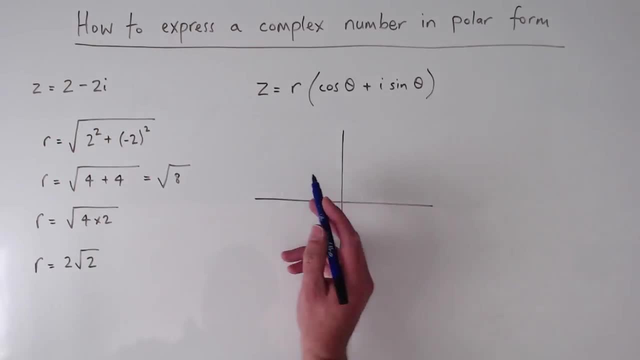 I was to plot 2 minus 2i on this axis. I've got 2, it's the real component in the positive direction, so that would be 2 there, and I've got minus 2i, So that would be down here somewhere. 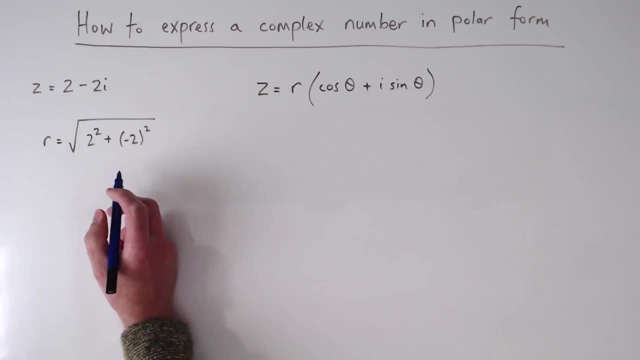 So it's plus minus 2 squared. okay, So if we work this through, that means that r would equal the square root of 4, 2 squared plus minus 2 squared plus 4.. So that equals the square root of 8.. Now to simplify this further, the square 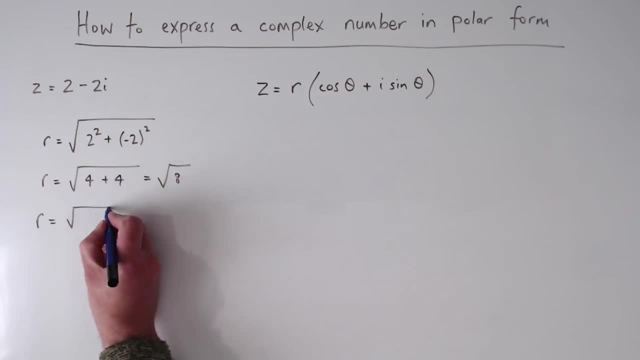 root of 8 can be written as 4 times 2.. I've done that because when I change the square root of 8 to 4 times 2, I have a square number here, so I can rewrite that as being r equals. 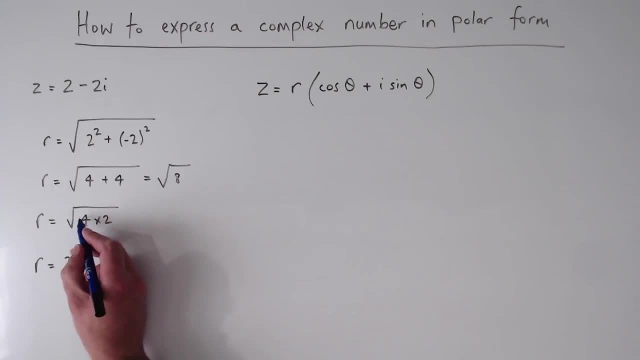 2.. We can take this square out: If here the square root of 4 is 2, 2 square root of 2.. Okay, So what we've done? by working out the modulus, we've got our first r component here. 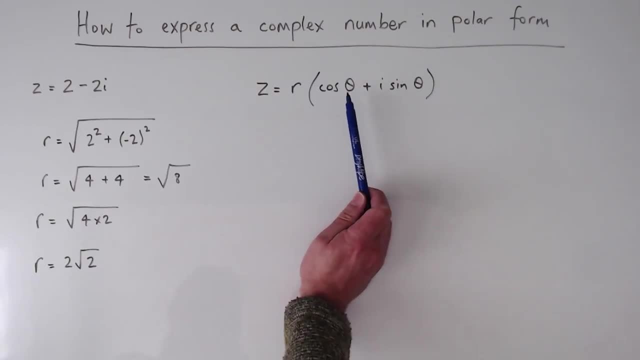 So we've done this part. We need to work out this angle, theta here, which they call the argument, And the way that we do. that is basically, if I have, if I, if I drew some axes, where this is the imaginary i-axis, this is my real component here. If 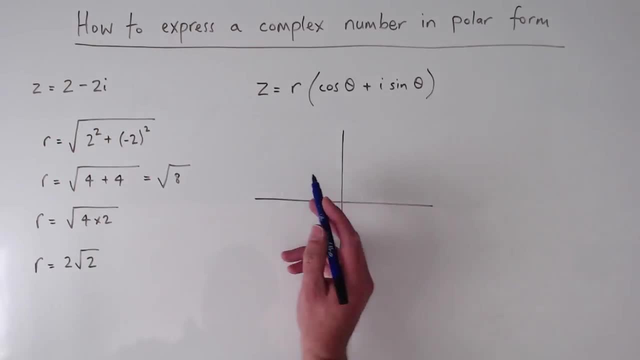 I was to plot 2 minus 2i on this axis. I've got 2, it's the real component in the positive direction, so that would be 2 there, and I've got minus 2i, So that would be down here somewhere. 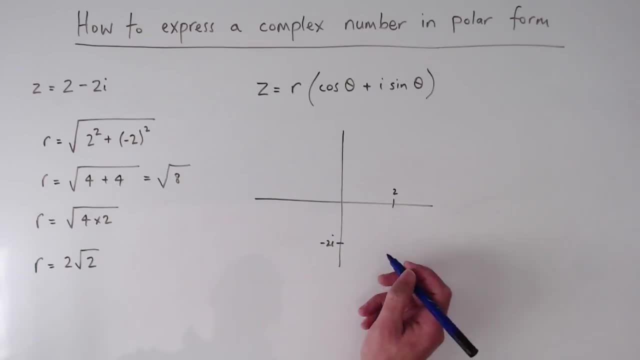 wouldn't it? This is my, my imaginary axis, So this complex number would plot here on this axis, And if I was to look at this angle here, theta, this would be the theta that we need to find for our code of form. Okay, Now, in thinking this through, we're going to think: 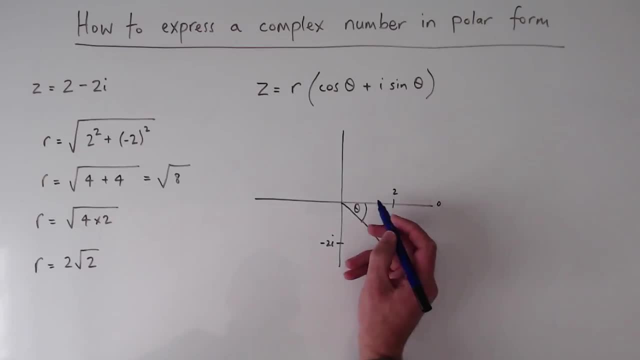 through angles in radians. We normally go from zero here, and if we go all the way around 180 degrees, that's called pi radians. When we're half radians, we're going to think through angles in radians. So if we go all the way around, that is a half of pi, which is pi over 2 radians. 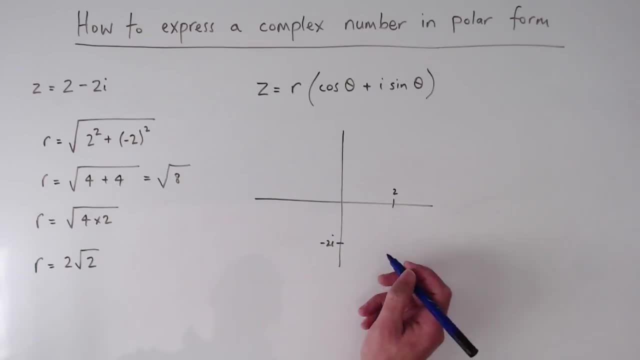 wouldn't it? This is my, my imaginary axis, So this complex number would plot here on this axis, And if I was to look at this angle here, theta, this would be the theta that we need to find for our code of form. Okay, Now, in thinking this through, we're going to think: 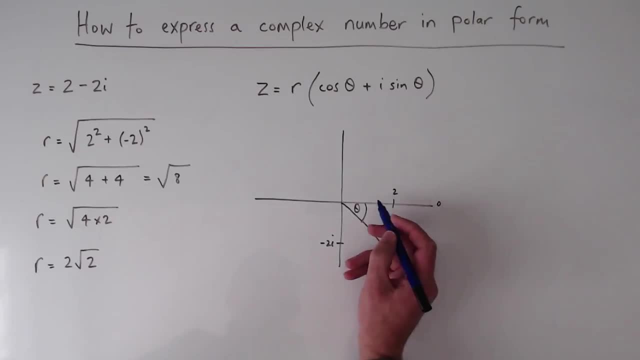 through angles in radians. We normally go from zero here, and if we go all the way around 180 degrees, that's called pi radians. When we're half radians, we're going to think through all the way around. that is a half of pi, which is pi over 2 radians. Okay, So angles are measured. 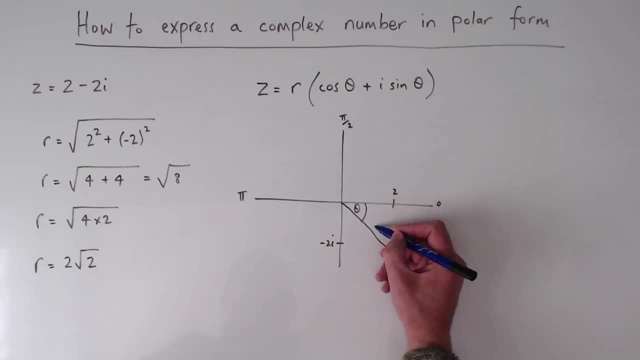 in this direction, but we're actually going in this direction in this case. So if we were going around in this direction, when we got to here we'd have minus pi radians, And here this is going to be. if we were going this way around, that would be minus pi over 2, if I was going 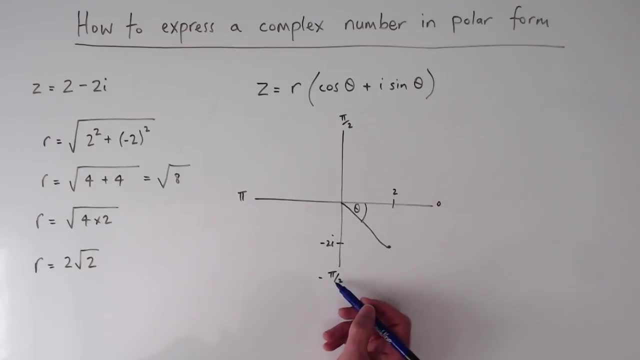 that way around. So that would be minus half a pi, but we're in between. Okay, We're actually looking at. anything in between is actually a quarter of a rotation. So this angle here is actually going to be minus pi over 4, because I've gone minus a quarter of a times round in my 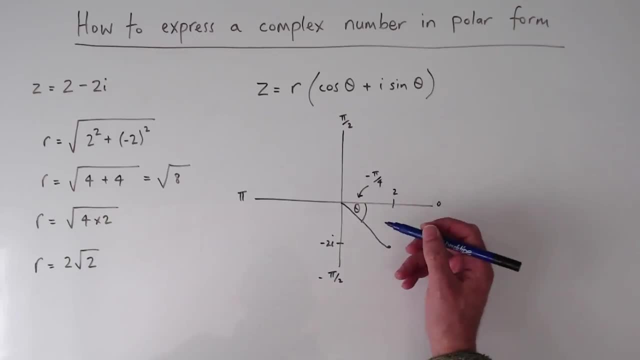 rotation. Okay, Now you could calculate that, because if we imagined that this was a triangle, then this distance here, the adjacent side- is 2, and this distance here is 2.. Okay, We've actually gone down minus 2.. So it's theta which actually equal the inverse tangent. 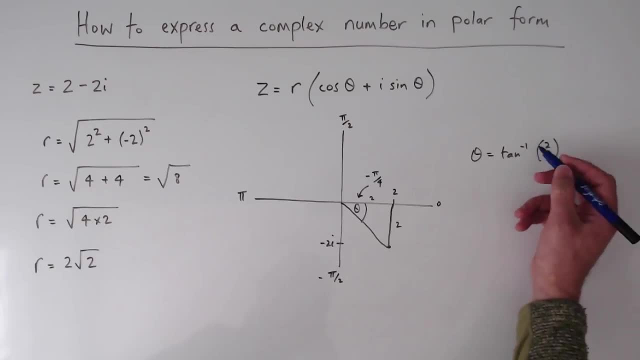 right of 2 over 2, which actually equals the inverse tangent of 1.. And on your calculator, if you work in radians, that will come out as pi over 4.. But because we've gone in an inverse direction, it actually equals minus pi over 4, because we've gone in the negative. 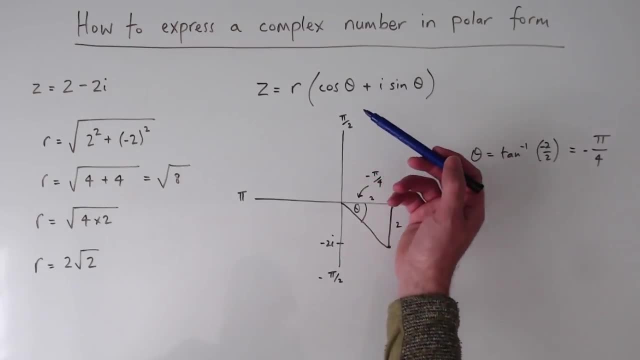 direction. So the theta angle. here you calculate it by plotting the real component and the imaginary component, as I've shown you, and either using the tangent rule, the tangent opposite divided by adjacent, to work out your theta in radians, or sometimes intuitively you 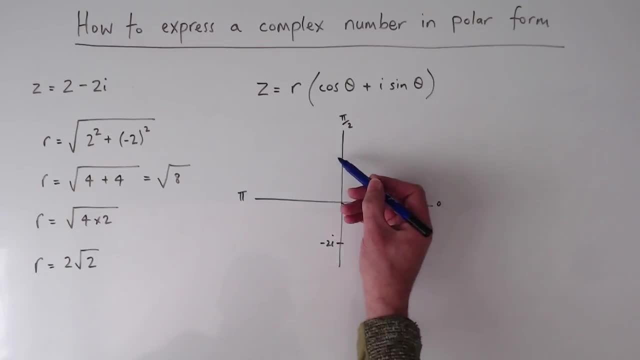 Okay, So angles are measured in this direction, but we're actually going in this direction in this case. So if we were going around in this direction, when we got to here we'd have minus pi radians, And here this is going to be. if we were going this way around, that would be minus. 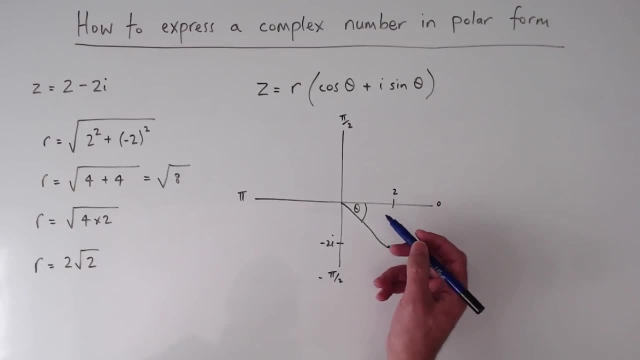 pi over 2, if I was going that way around, So that'd be minus half a pi, but we're in between, Okay, We're actually looking at. anything in between is actually a quarter of a rotation. So this angle here is actually going to be minus pi over 4,. 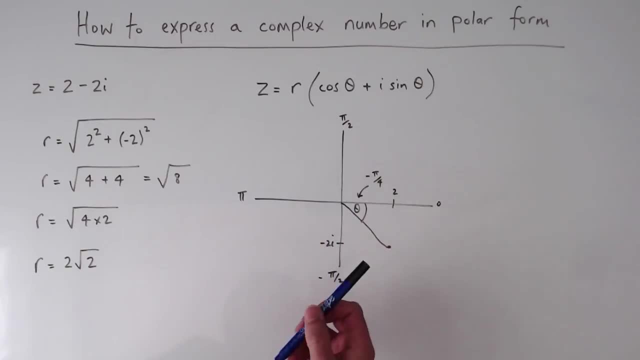 because I've gone minus a quarter of a times round in my rotation. Okay, Now you could calculate that, because if we imagine that this was a triangle, then this distance here, the adjacent side, is 2.. And this distance here is 2.. Okay, We've actually gone down minus 2.. 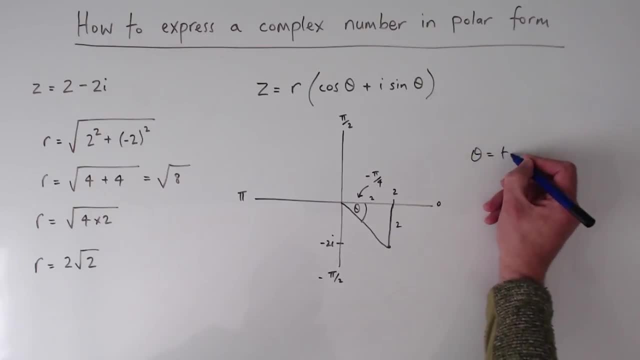 So it's theta which actually equal the inverse tangent right of 2 over 2, which actually equals the inverse tangent of 1.. And on your calculator, if you work in radians, that will come out as pi over 4.. But because we've gone in an inverse 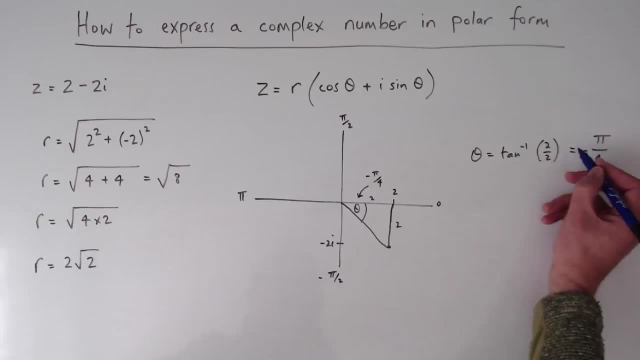 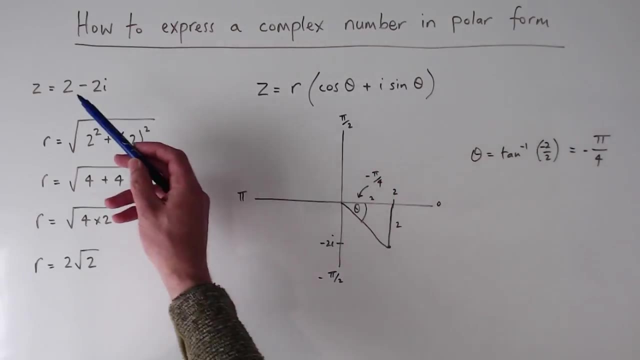 direction. it actually equals minus pi over 4, because we've gone in the negative direction. So the theta angle: here you calculate it by plotting the real component and the imaginary component, as I've shown you, and either using the tangent rule, tangent opposite divided by adjacent. 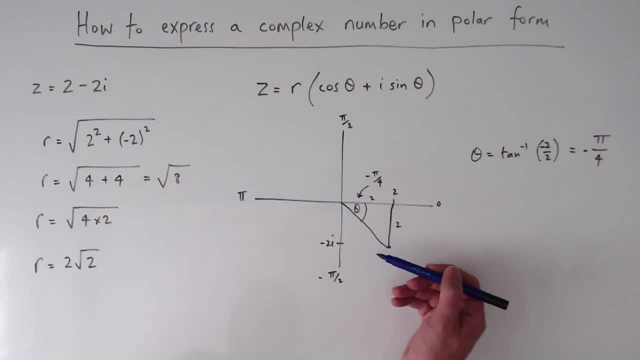 to work out your theta in radians, or sometimes intuitively. you can just think: in this case I just did a quarter of a turn. in this case I just did a quarter of a turn, So I knew I'd gone minus a quarter of a turn.